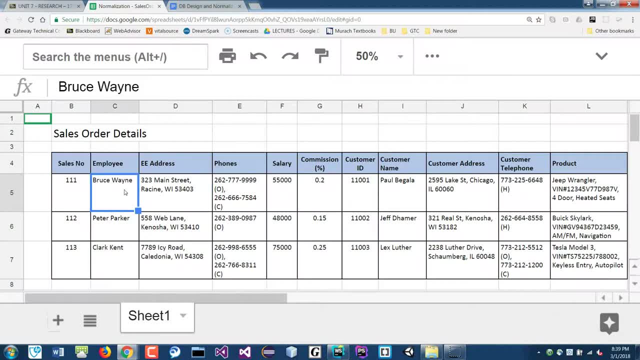 Okay. so this is okay. this is okay because it's not multi-value. I could, if I have like Bruce Wayne comma, you know, You know Joe Lang or something, then that's multi-value right. 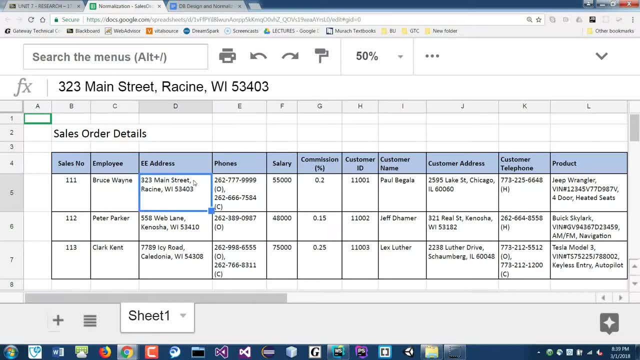 So that's fine for this column. What about this one here? Yeah, it is multiple right, Or you can well actually. yeah it is it is. You can break it down into four columns or three columns. 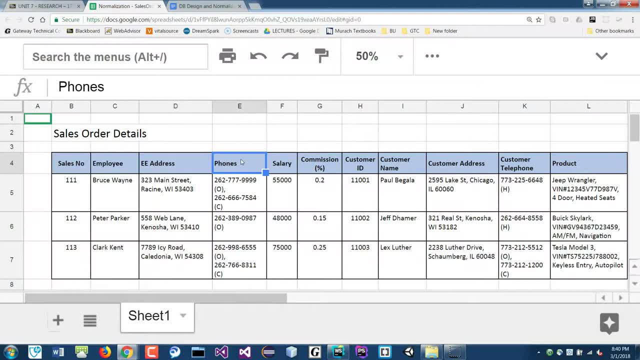 So you need to break that out. Phone numbers Also multiple, So you can see that I failed already, right, So anyway, so that's good, You need to break that out, this out. This is okay. 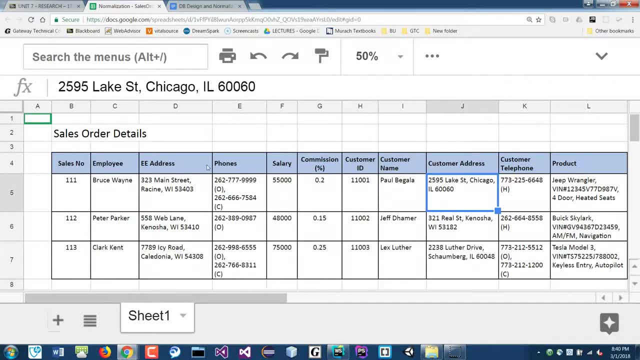 This is okay. The address again same thing as over here, So you can break that out. This one also failed because one has two numbers here same thing And then the product That also had multiple. So those columns failed. 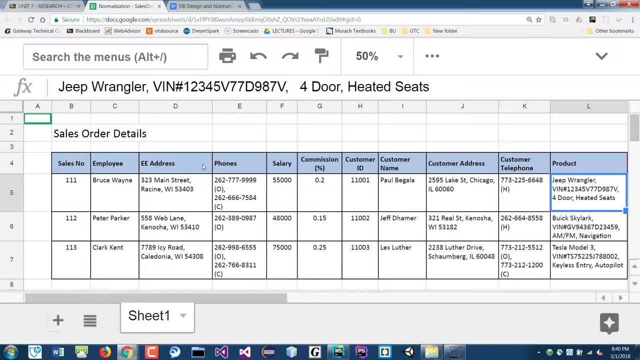 So So what should we do here? So we can add columns, additional columns for the address, the street name, the city, the zip and the state. Or you can say we can take this employee information out. All these are about the employee here. 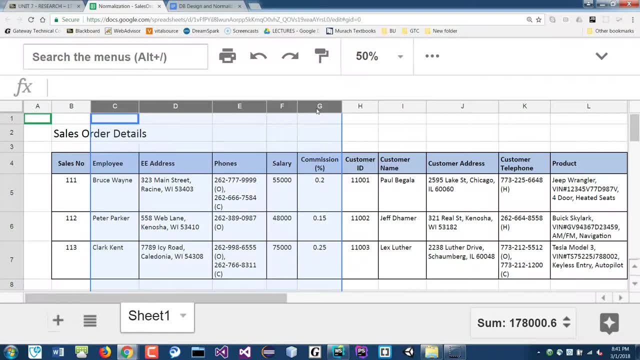 These, these columns here, right, And then we can take that whole thing out and make its own separate table. okay. So if I do that, if I say take the whole row out or columns out, and if I were to, it's kind of hard to do here. but 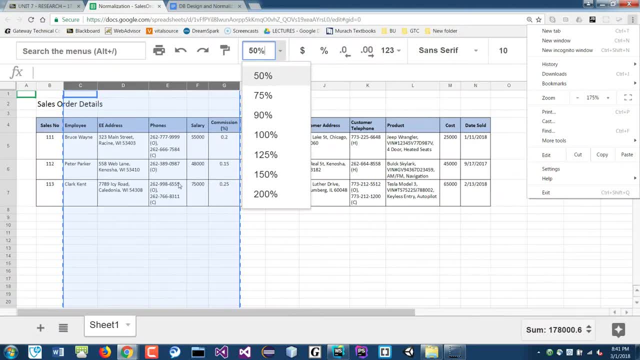 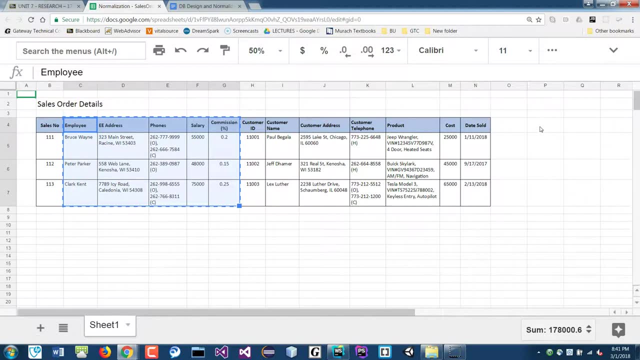 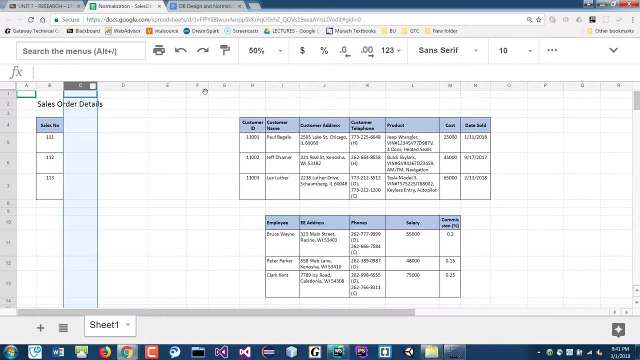 So what should? what should go in its place? Let's do it again If I take these out And put it over here, Somewhere over here. Okay, So, Yeah, right, So we can. we can replace these with the employee ID. 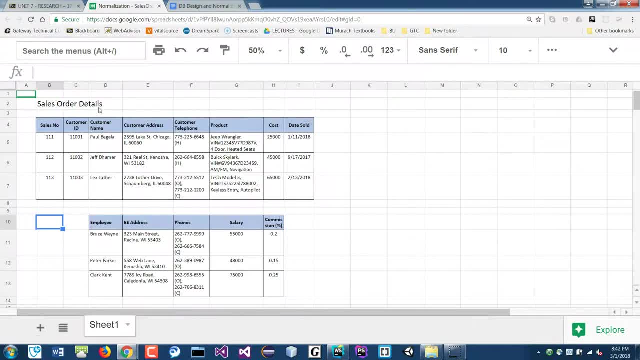 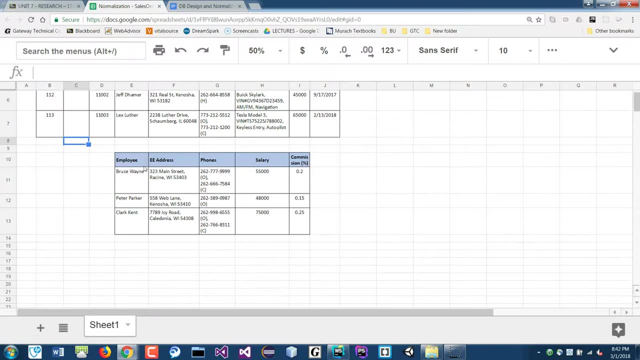 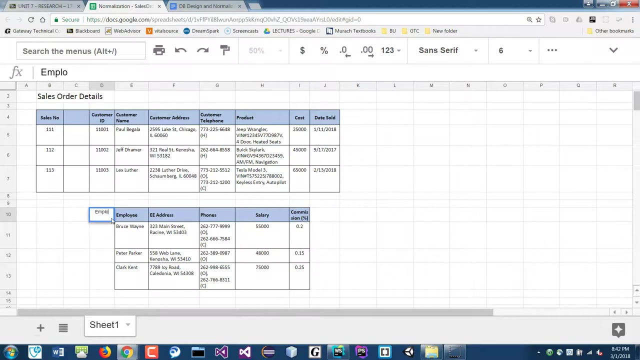 Let me add that additional column here Insert just one column to the left of this. So here we need to put an employee ID here, And so we can add another column employee in here, And this could take 1,, 2, and 3, and 4.. 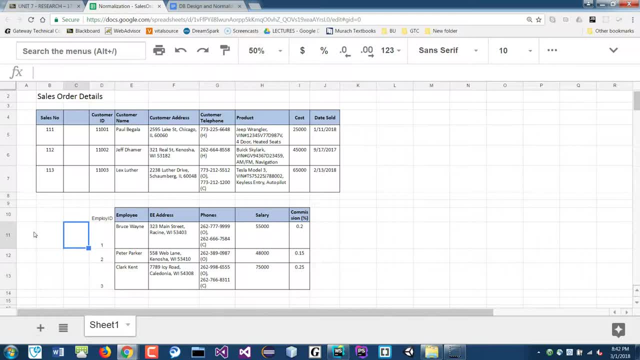 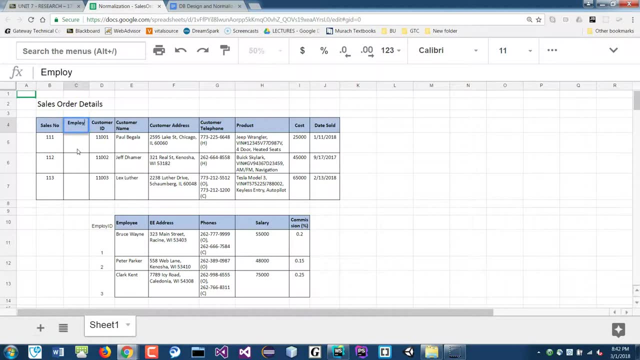 However, you want to choose it, to use it right. It could be numbers, It could be something else, So it's up to you. And then in here we'll make this as the foreign key And we'll make this the FK here. 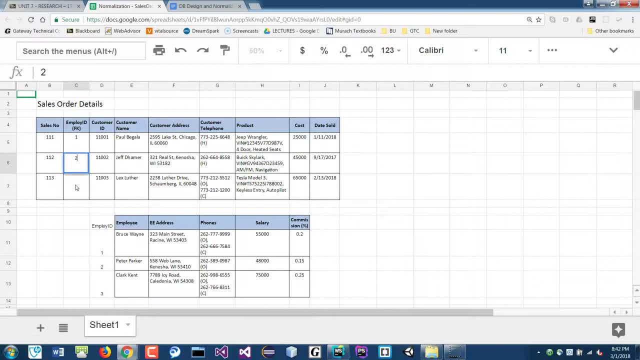 And then this could be for Bruce, This is Peter And this is Clark. Okay, So now this one is unique. Well, it's all about employees, So that one is good. And then here we have this address here, right? 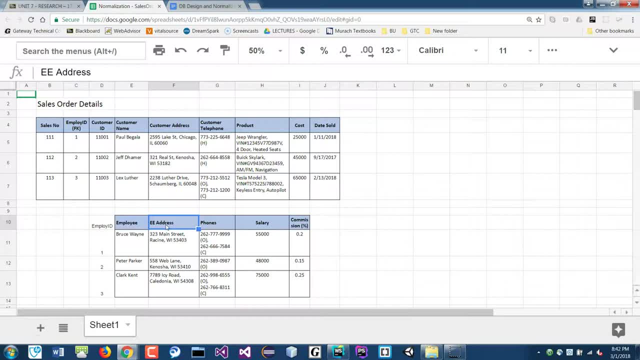 It still fails that first normal form. So we have to break this out And send it to the phone number And to their own separate columns. So let me just, you know, cut this, Put it over here, Let's see. 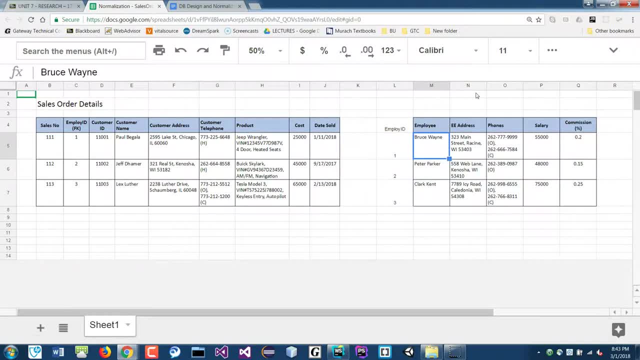 Okay, so that means that I could break this into the address And they have the you know city And then state and zip and so on, right And then state, zip And the phone number. the same thing. 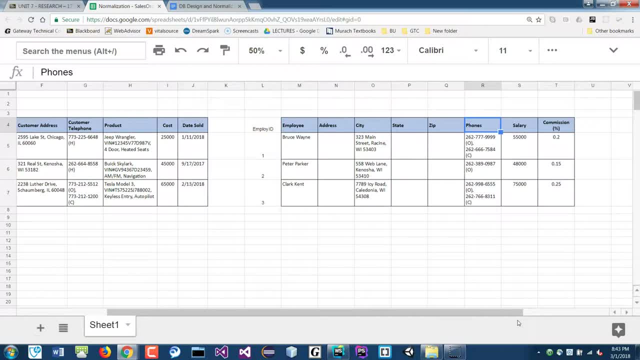 Okay, So I'm going to put this into two columns, Just so you meet the rule. You can say: here phone one And then phone two, right, And I'm not going to put data over it, But that's what we get. 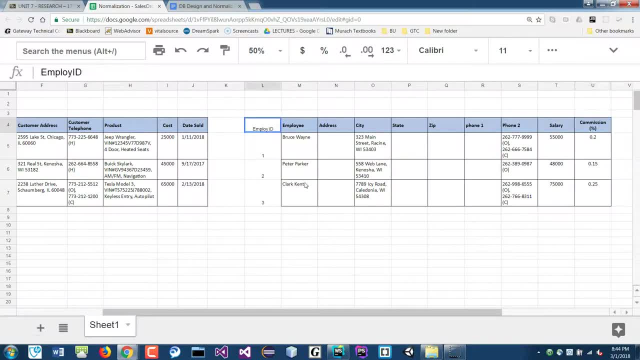 And this is by itself, by itself, So you're good. So this table here now meets the first normal form right. It has a primary key. This would be the PK. So also a first name and last name. 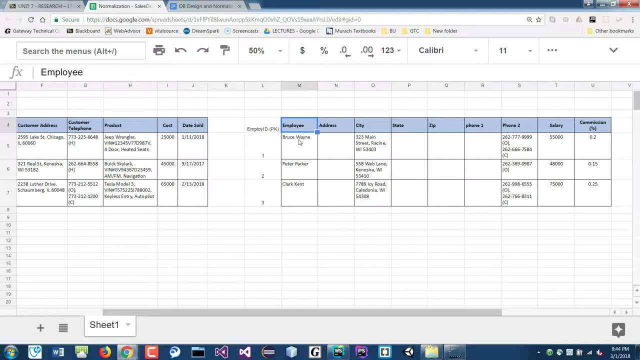 Well, actually here, you can leave it as is Or, just to make it better, you can break this into first name and last name. okay, Usually that's the preferred way, But agencies violate the first rule. It's just that it looks better that way. 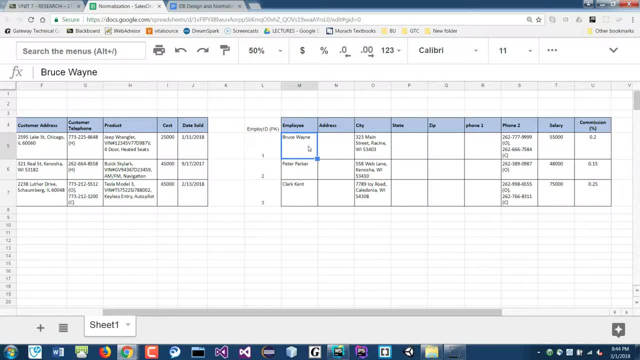 It's also easier if you want to sort and search data. It's better to have its own column, So you can break that into first name and last name here, And it's all good, right, And so the first number four is fine. how about this table over here? 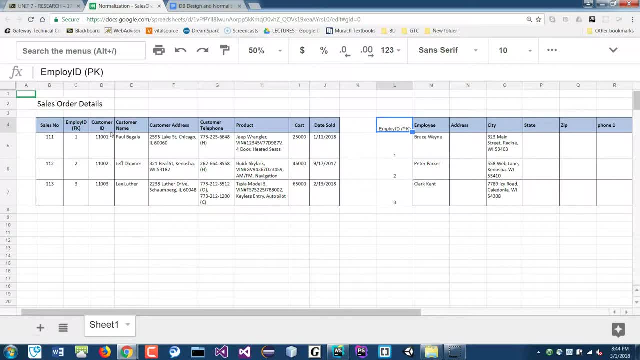 Once you take that out, you have to consider this one too. So again, we have the same stuff, We have the customer information here. okay, So I can do the same thing, right? You take all this customer information and you take that out and put over here on the 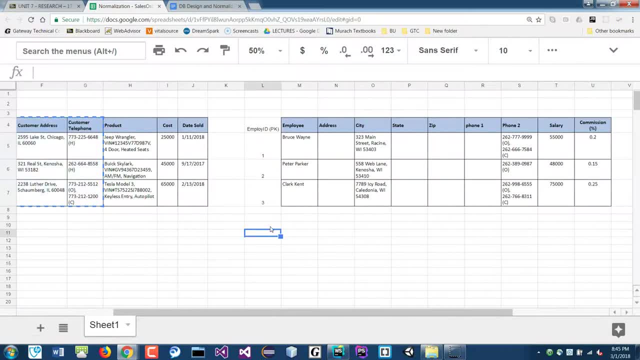 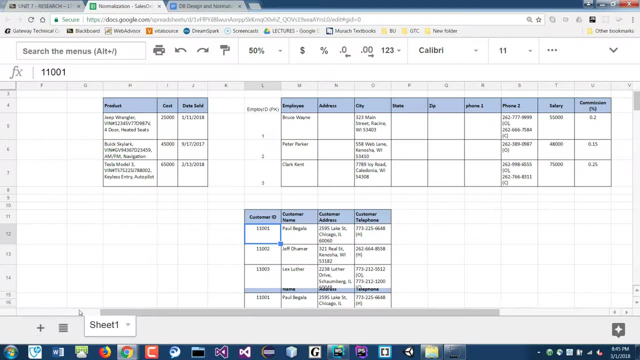 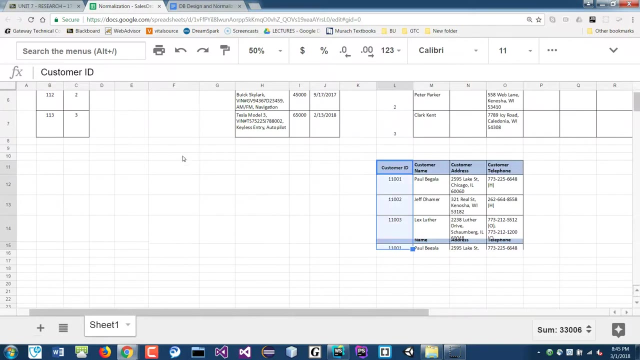 far side in here. we'll put the customer table over here. I have the customer ID already. that's good, And then on the original table I will leave the customer table column as it was before. We'll make this the foreign key right. 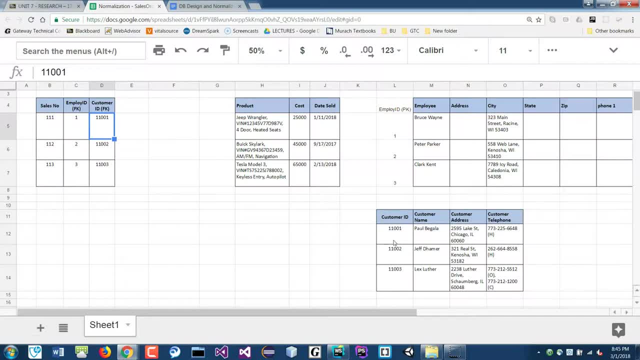 So again, it's linked to this customer Because one customer, Okay, So we have. So if you look at the employee table here, why did I put this as foreign key? and this is the primary key and not the other way around? 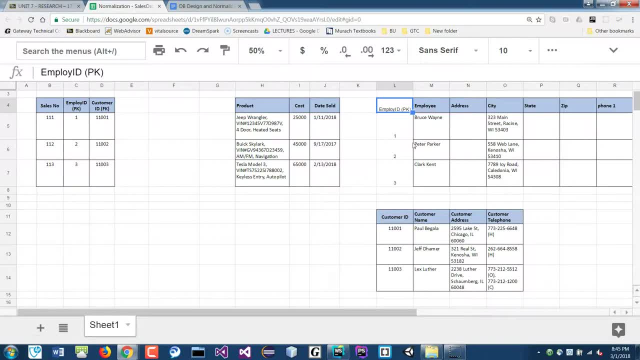 Yeah, the same thing here. Why do you put this as foreign key? and this is the primary key. So Go ahead, Your sales order, your Yeah Yeah, Yeah, Yeah, Yeah Yeah, And your sales table. the primary key is your sales order. 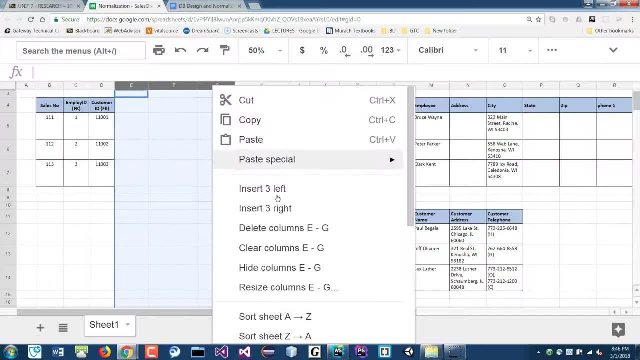 And that's all the entries in there. It's a part about sales, and then you're referencing customers or you're referencing the employee numbers. Yes, Yeah, Whenever you're referencing those, those are foreign keys. Yeah, Yeah, Right, That is correct. 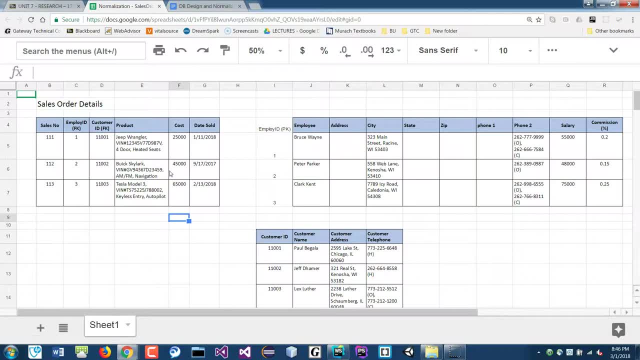 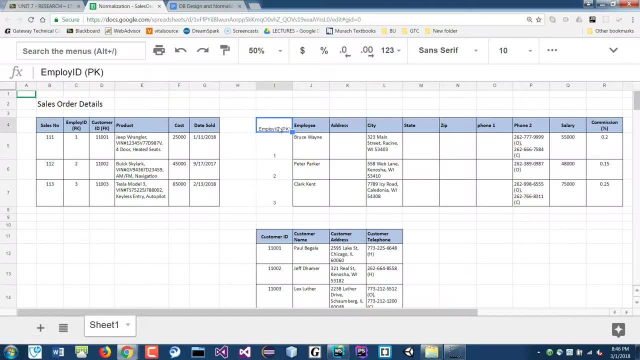 Why did you decide that the foreign key is here and not over here? Why, ok, not? Why don't I put it sales as the foreign key over here? You know what I mean, Because the unique ID in the sales order details table is the sales number. 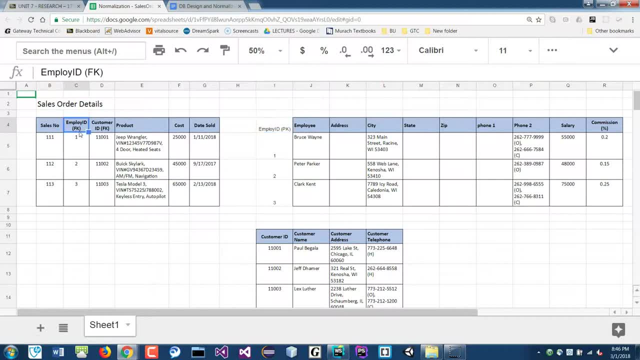 There's only one sales number- that if going to be 1-1-1,, whereas the employee ID number 1 can have multiple sales in that sales table, of course. Okay, So sales in that same table. Yeah, I think you got the idea. 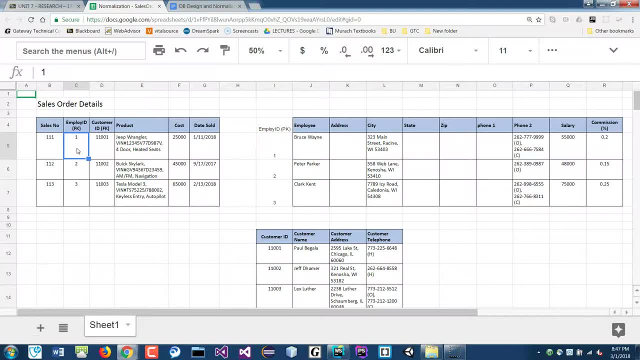 When you look at the employee table, there's only one employee, number one. so that is unique value there. Right, Right, you are absolutely right. So you think about relationships, business models here. So you think about it this way. 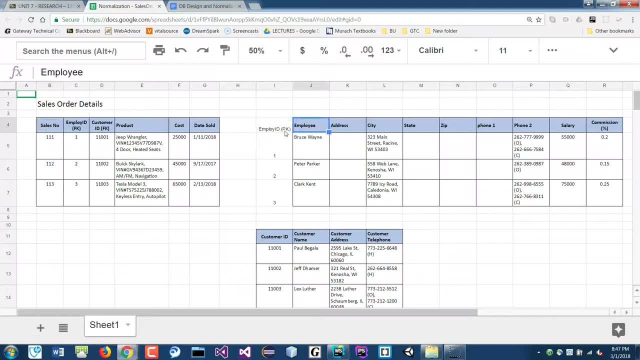 I have a sales order. I have an employee Now, so as an employee you can have many sales orders. okay, So I can sell one car, this order for one customer. I can sell the same customer. I can sell another car. 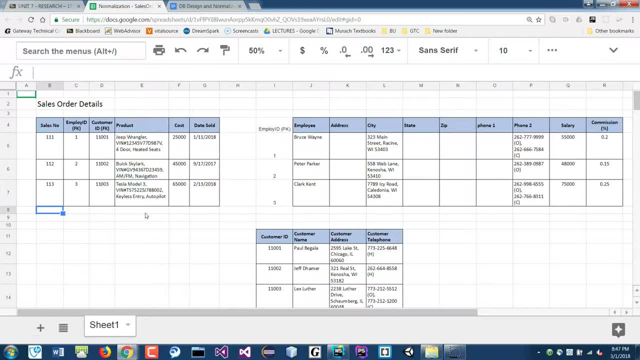 with the order number 114 to the same customer again or a different customer, doesn't matter. So if you look at this, one employee has many orders, So that's why the one is always the primary key. The main side is the foreign key. 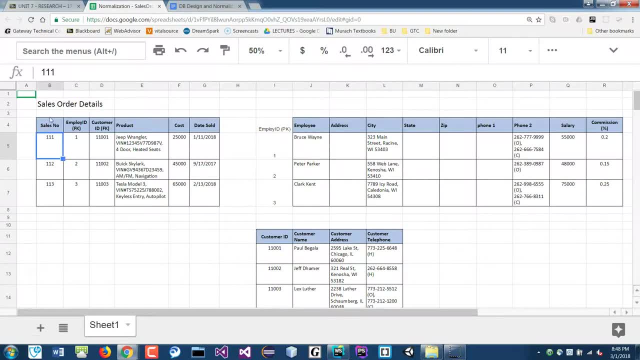 Okay, it doesn't make sense to go the other way around. A sales order can have many employees. So in other words, I guess- unless you allow it, right, but usually you have- one order is sold to one person by one person. 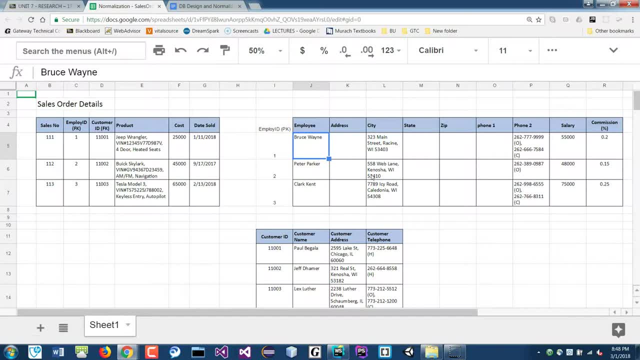 Okay, unless you have a dealership that allows. you know two or three people here can sell to one individual and you co-share the pay. I guess. If that's okay, then we have a many-to-many relationship, okay, Okay. 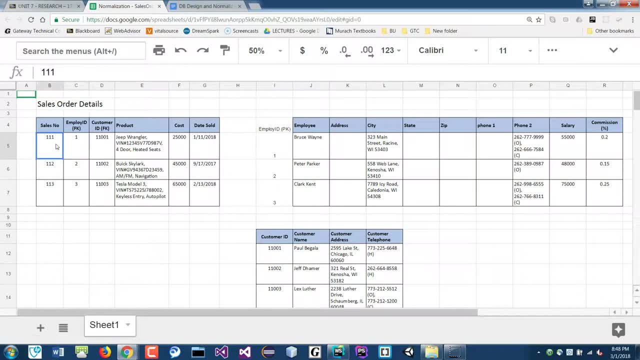 But in this example it would be like a one-to-many Same thing here. right, The customer can be a client. Well, yeah, a customer has one order or have many orders. right, I mean, I could buy one car. 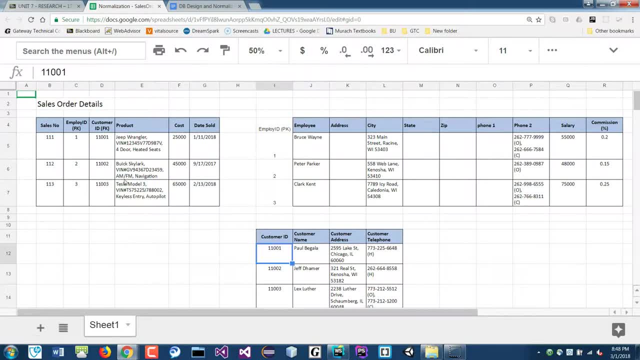 from this dealer, or I can buy a lot of cars from this dealer in the next you know month or next year I could come back and buy it again. But one order here is usually very unique to only one customer, okay. 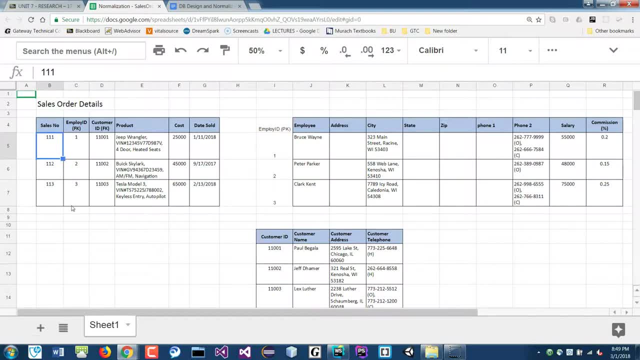 So again, you have the one-to-many relationships here, So again. so that's why we put the foreign key here, And so usually, if you think about this, that's how it is, Or the easiest way is basically, every time you take out some data. 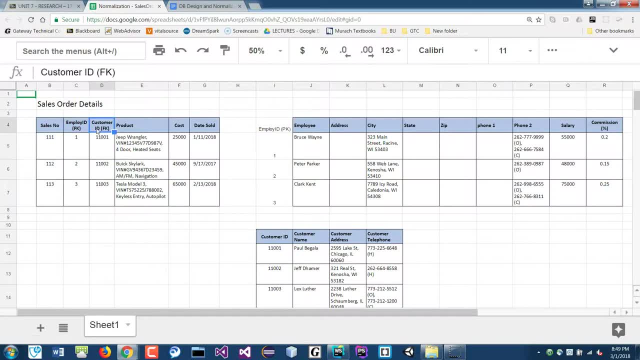 out of this big table. these are usually the foreign keys. okay, You end up asking the foreign key because you take something out of it and you can link it back to that as the foreign key, And sometimes you don't have it at all. 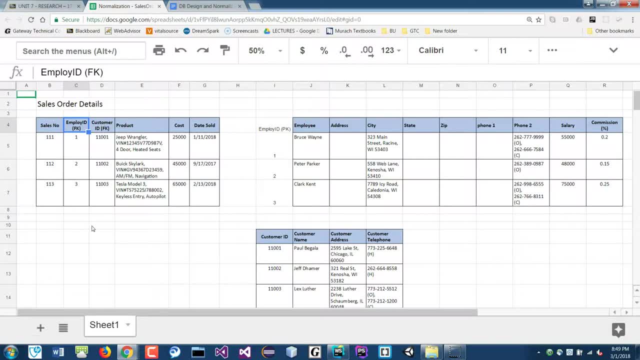 because you might have. you might remove this table completely and you build a different table out of that, so you have to also consider that too. But usually when you take it out from this big table, you have a foreign key in there, okay. 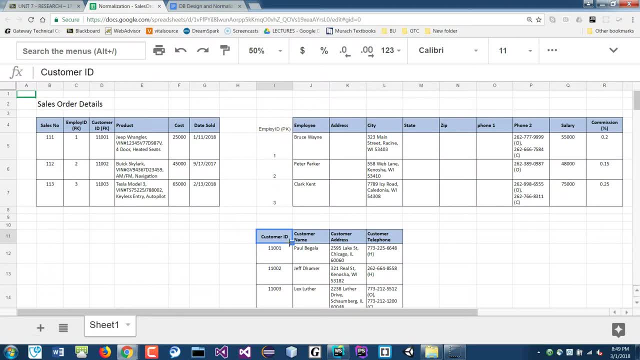 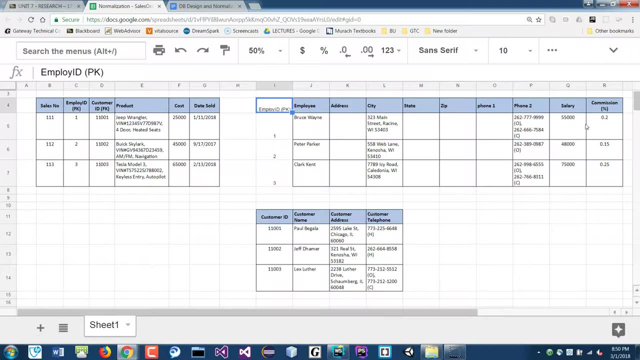 So now this customer table here is not first normal form, because we have the addresses and so on the phone too, So we can break this. it will look something just like this one here: Okay, It's the same rule. Once you do that. 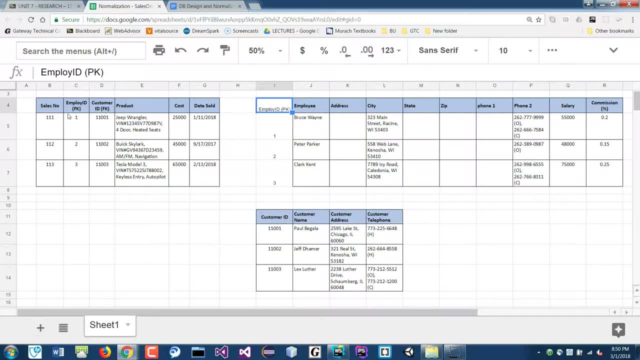 then it qualifies, it meets the first normal form and then this one. here we still have things to do. So we have the products information here, right, So you can break it down to each columns. Maybe you have the Jeep, it's like a make, right? 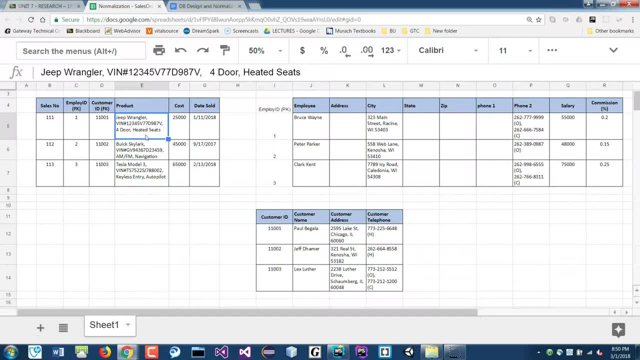 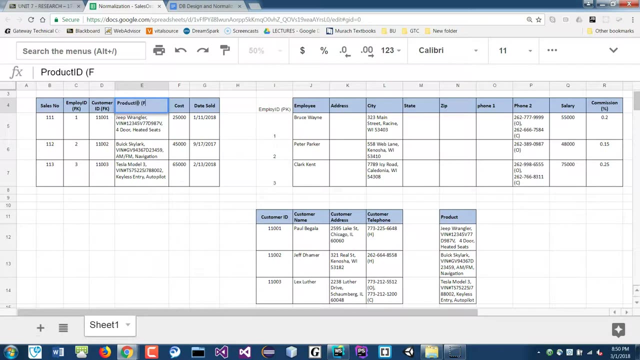 Make model, VIN number and then the descriptions or the features here. So again you could take this whole thing out and put it into its own table and then here you put the product key, right ID, and then you bring that to the foreign key. 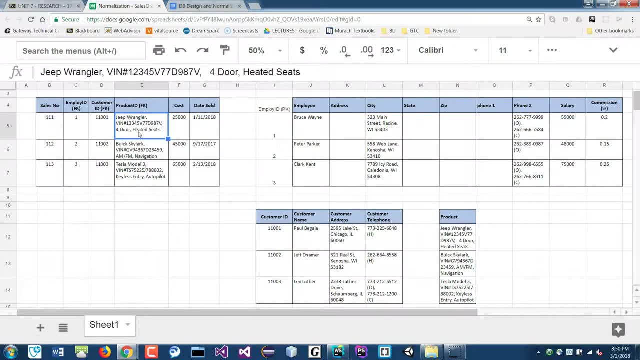 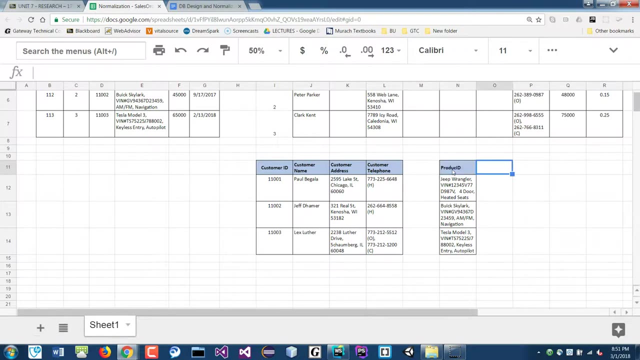 And here you just put: maybe you can use the VIN number as the key. Okay, So over here you have this table of products. This could be the product ID, and then you have the make model and then we have the features. 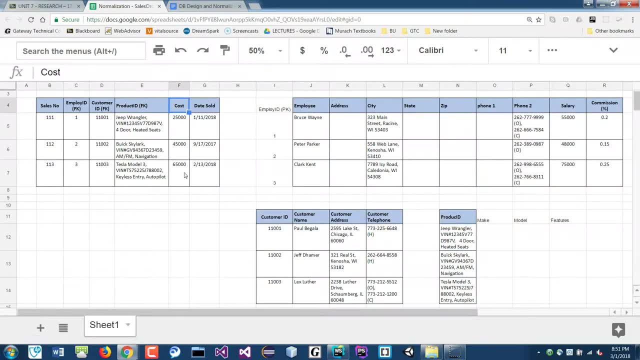 And then maybe the cost as well, the cost of the car, Okay, So that could also be taken out and added to the product table. So you put Jeep and then a Wrangler. no, I mean, sorry, it's the VIN number. 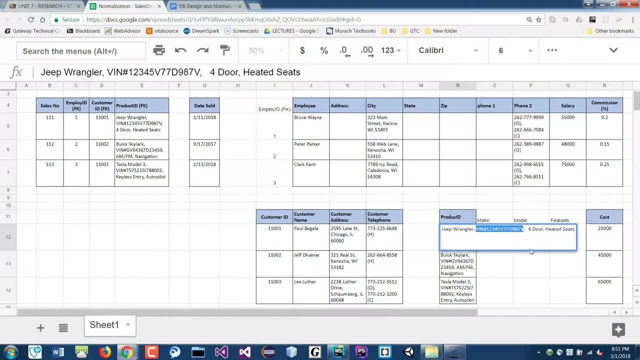 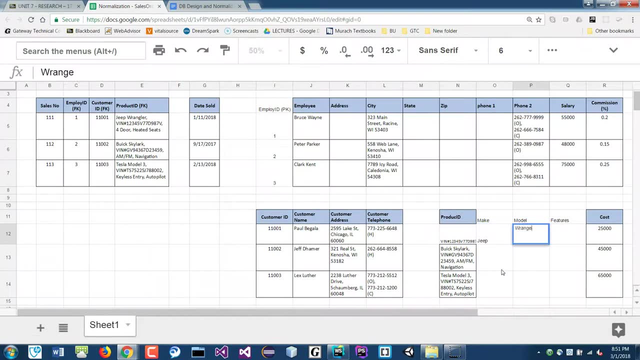 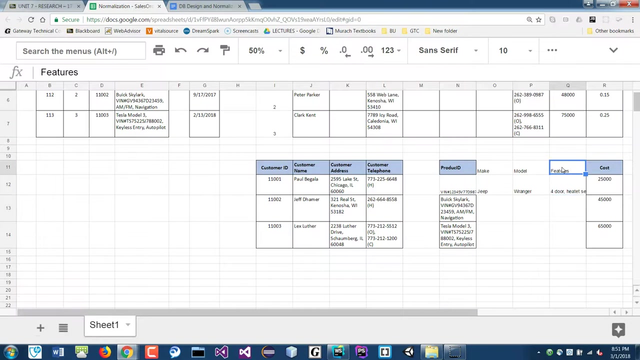 It's number. here This would be the VIN number. You can use that as the ID. And then we have the make: it would be Jeep Wrangler, And then the description: we have four-door heated seats. So here we have another problem. 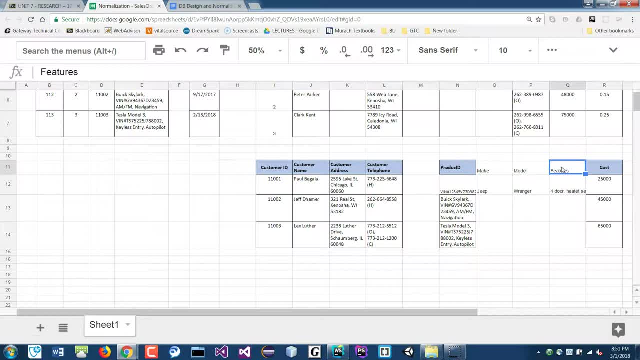 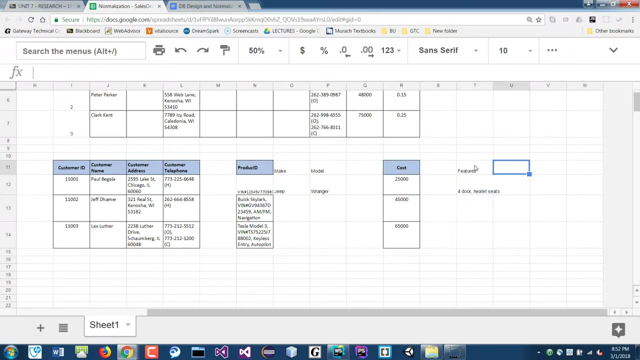 The feature is not normalized Right. It fails that second rule, So you have to break it down into a separate column Again so you can take this out into another table. You can see how fun this gets right, So put a feature over here. 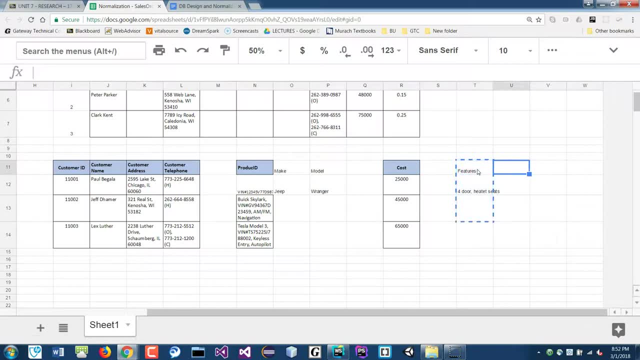 Let's put it over here, And I have here a feature ID Could be one. Here we just four-door. Two will be the heated seats. Right, You get the idea right And you can see all the other cars has it too, right. 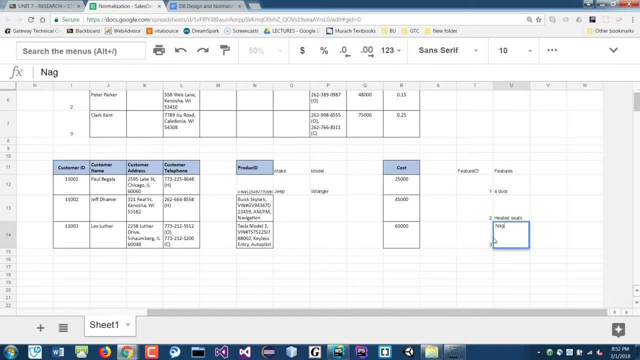 You have the navigation, so three could be for navigation and so on. So each has their own data. And then, since this is the feature ID, we took it from here, then I have the feature ID here as the foreign key And it will be linked to one. 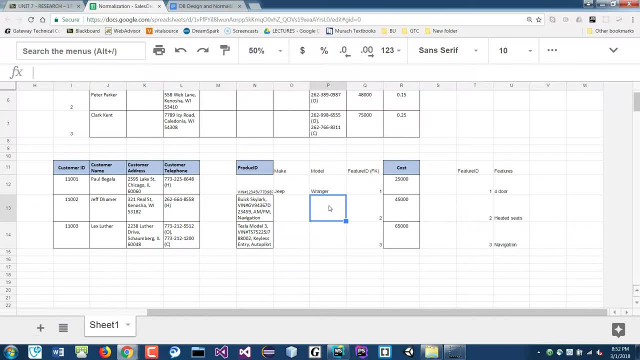 to two and three and so on. Okay, So you got the idea. So now that qualifies as the first normal form. The other one is completely normal form. This is actually already in third normal form. We actually, since we have a- 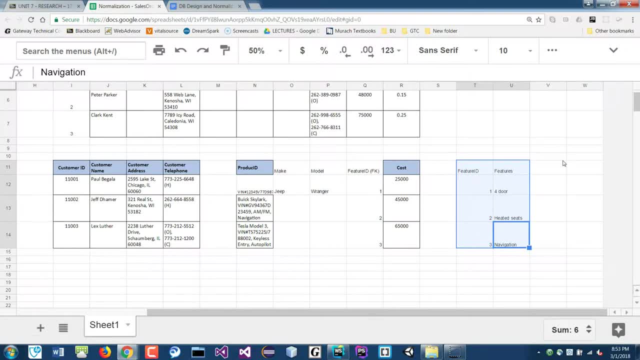 any time we have like a really short column like this- one or two or three columns usually- that can be easily converted to the third normal form, Even the fifth or sixth normal form by default, because it's just so simple. Okay, So this is good. 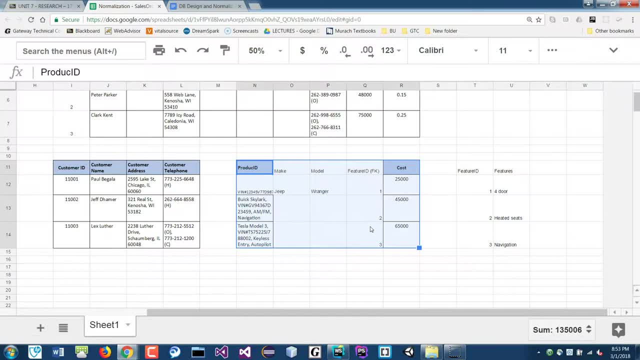 This is good. The features have been confused. The feature Yes, Because what if product ID and that VIN number has multiple features? Oh yeah, you're right. Then what? So you have to go feature one, feature two and 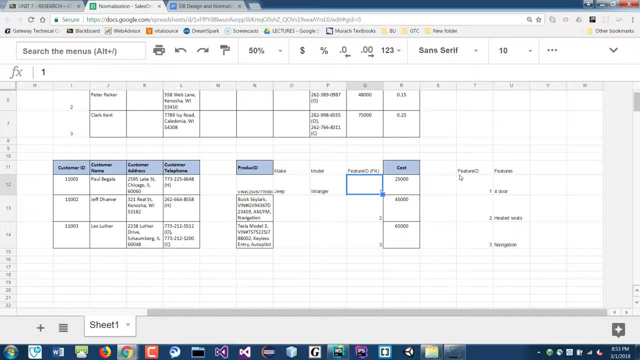 Mm-hmm. Yeah, Right, So You created the table of packages, right? Feature packages or something like that. Yeah, Yeah, Okay, So great, great. I'm glad you asked that, because I didn't catch this. 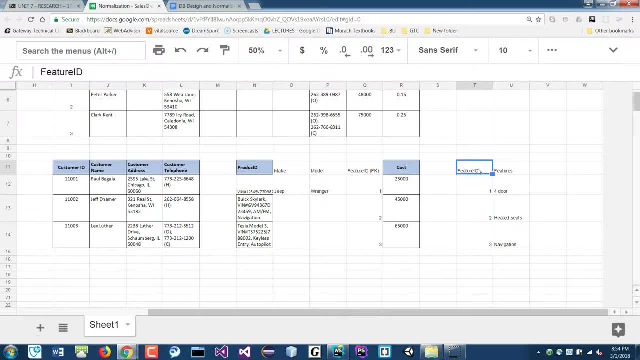 So The features have to be in different rows. Yeah, Yeah, So feature number one has this door package and this seat package, Mm-hmm, Something like that. Yes, Yeah, Perfect, Yeah, And I'll let you get a package. 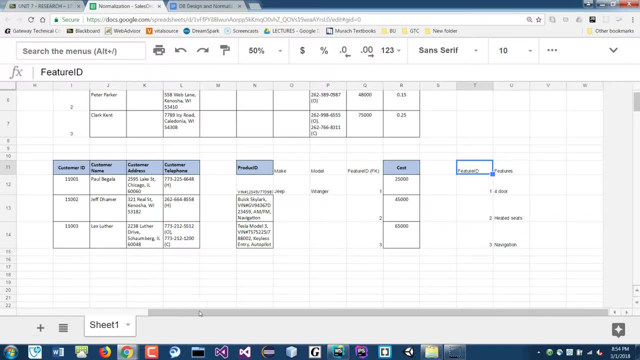 and I'll let you get a package, and I'll let you get a package, Yeah, Yeah. So this is, This is an example of a. So Okay, Let's look about these two tables here. Let's look at the product. 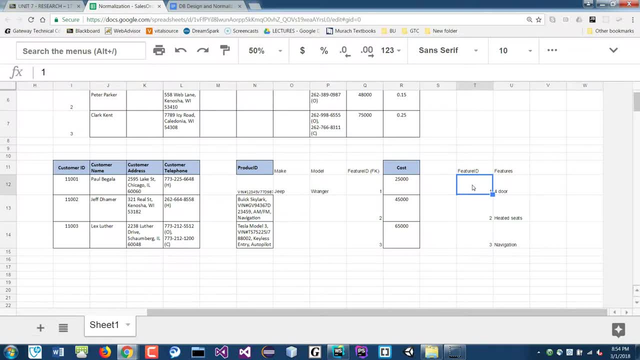 and the features. So a car, the Wrangler, Can a car have more than one feature? You can right. Can one feature be applied to more than one car? Yeah, Yeah, So we have a many, many two relationship here. 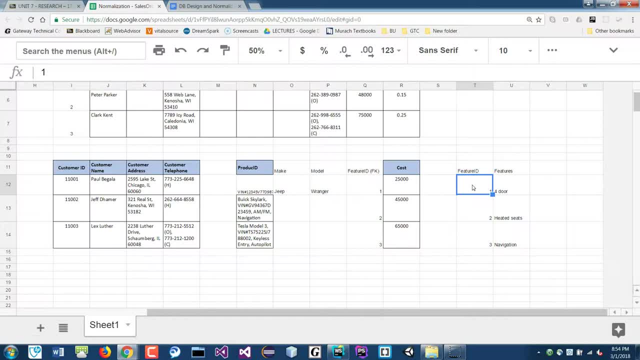 Okay, So we Now this brought to the example, Okay, Okay, Okay, So to make this work, because if you don't do this, I will have to list this X number of times just to show a different feature for this ID. 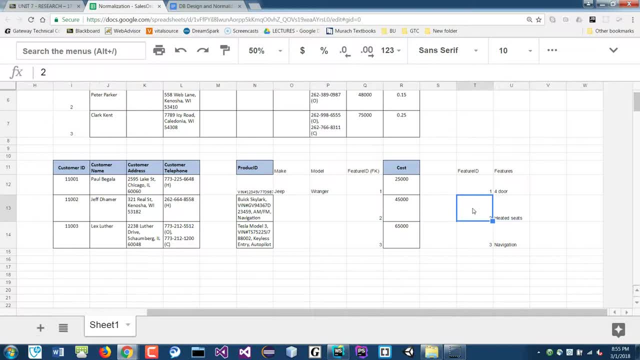 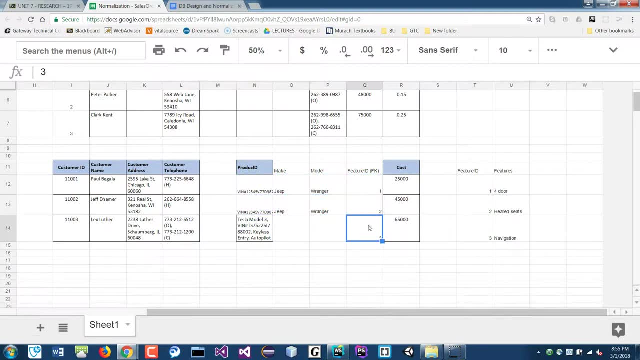 I could list this again. for example, I might do that here and then show feature two. And now, if I do this, this is no longer unique, So I have to have another ID here to track the Each individual car here, which is: 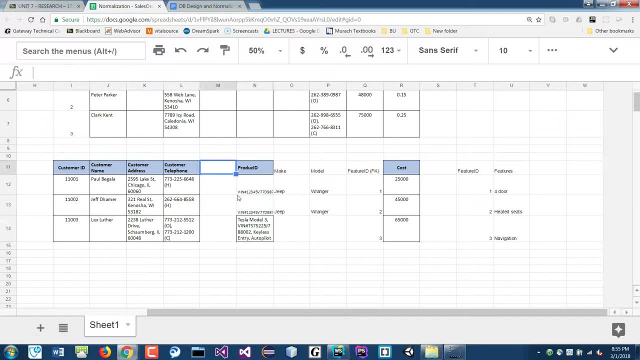 Makes a lot of Problem, right? So I have to have another ID here to track the Each individual car here, which is Makes a lot of Problem, right? So what you have here is what's called a many-to-many relationship. 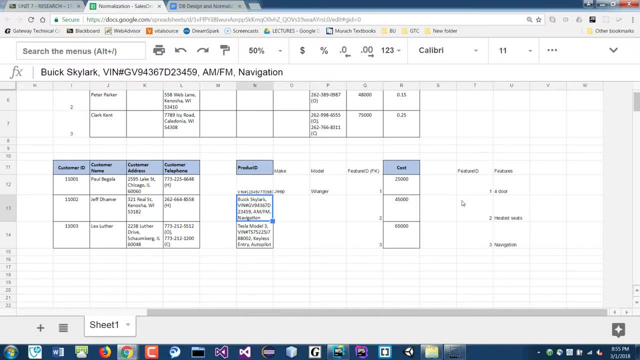 And I'm glad you caught that, Julie, so thank you. So now what you do is you have to have a junction table between this and the product table to make this work, Okay, So let me copy this And we'll move it over here. 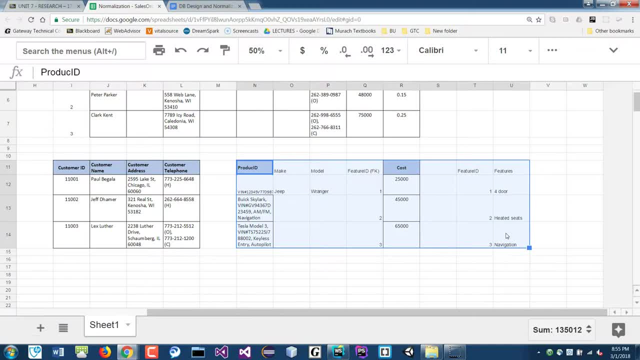 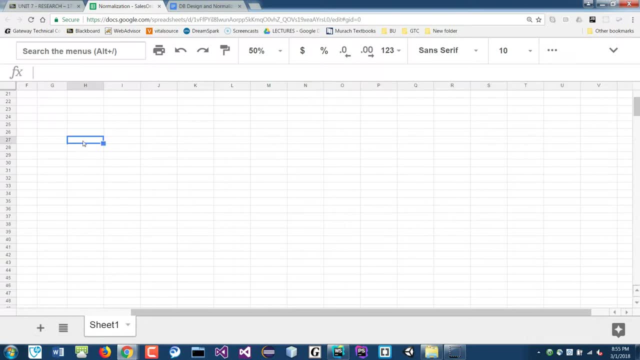 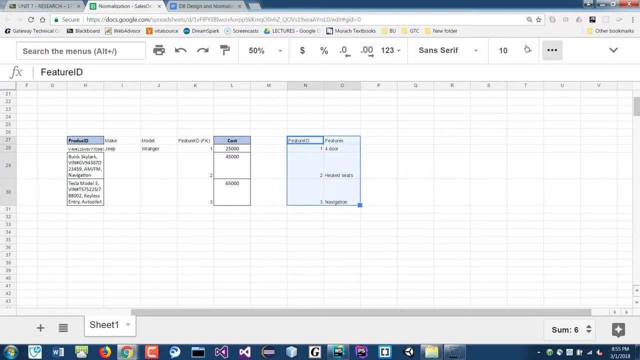 so I have more space. Let's put it over here. Okay, So I have the feature and the product here. Okay So I have the feature and the product here. Okay So I have the feature and the feature table here And let me just. 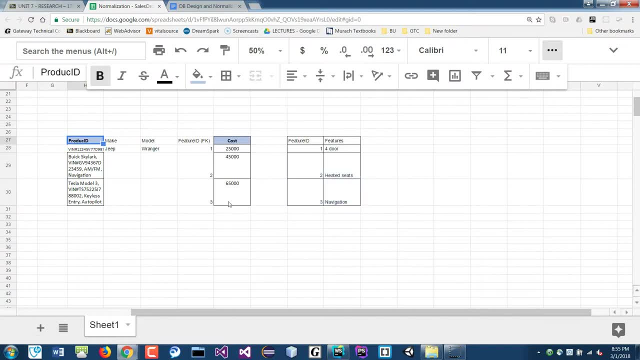 put that here We have the product. Okay, This is a. So when you build a many-to-many relationship, you have to have a junction table. So here I have. I'm going to move this a little bit on the other side. 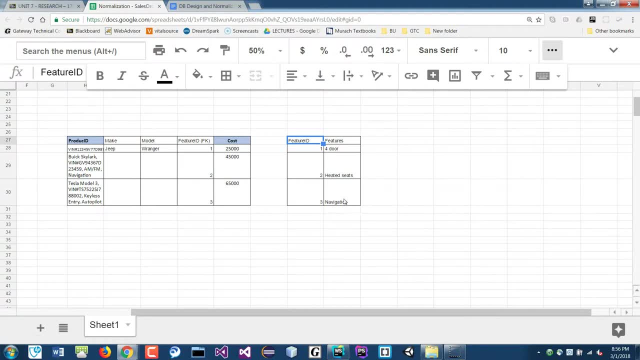 over here. Okay, I'm going to have another table in here which will have the product ID and the product table here. Okay, So I have the feature and the product table here. Okay, So I have the product ID. Also have related to: 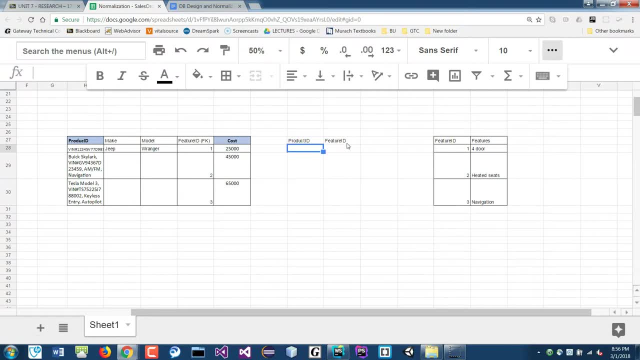 the feature ID. Okay, So this is the junction table that can link the two, And this is what's needed if you want to build a one, a many-to-many relationship. So now I can put the product ID in here. Okay, So I have. 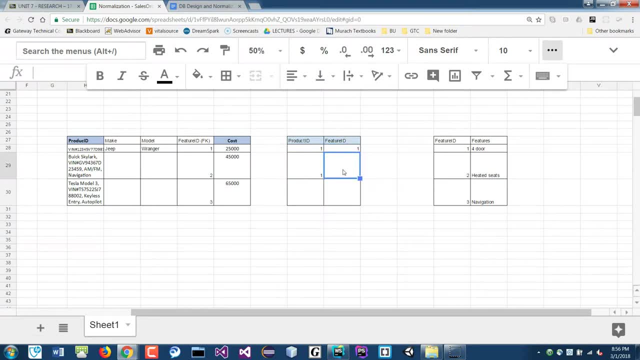 another one of these and I can put it in the other one and I can put it in the other one. Okay, So now I can put in that product ID and this one would be a. So I have all of these here, So I can. 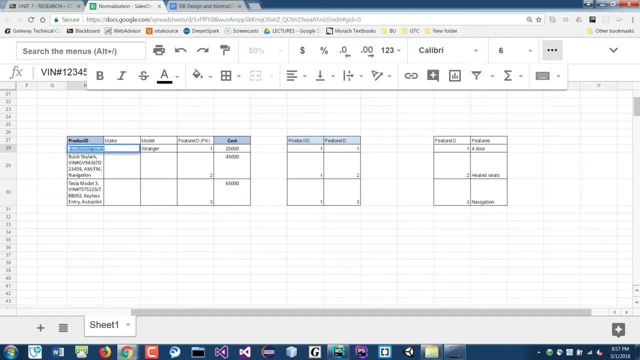 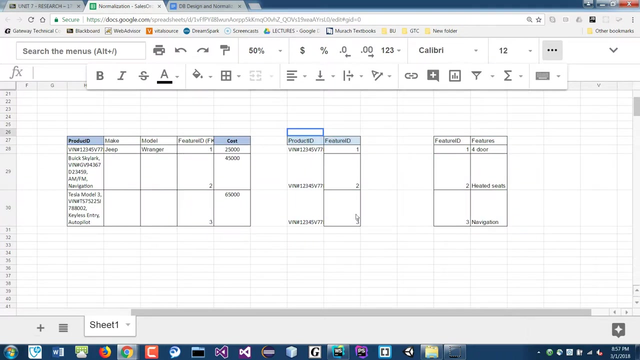 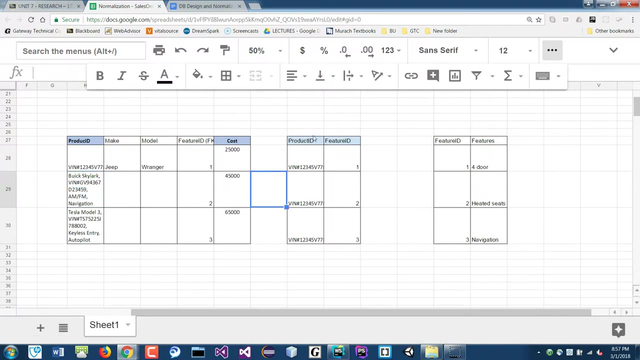 put this yet yet, so they remember. so, uh, but i can, and i think it's not worth much better, okay, so right, you have to be a member and let me just uh increase, okay, so this idea here is the foreign key for this table here. 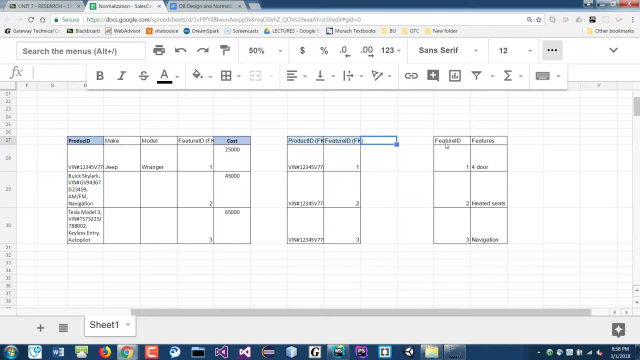 and this is the foreign key from this table here. so if i say, uh, give me the car, it has a priority of the number of this. it has uh then then then join right, join this to have the uh would have matching of product id in this table. 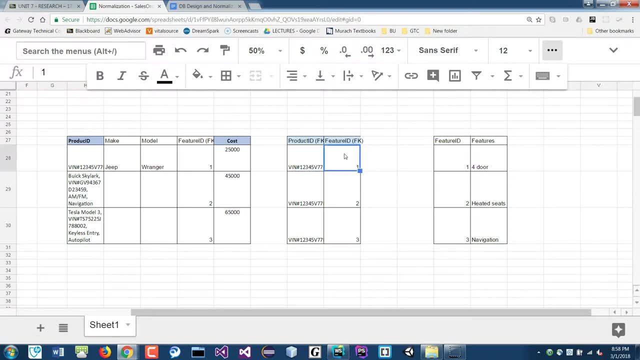 and join this table here with the matching key of this. so if you look at this, you see that this bin number here belongs to this car, jeep, and it has three features. okay, and all these three features here. uh, described a single car, but this is this column here. 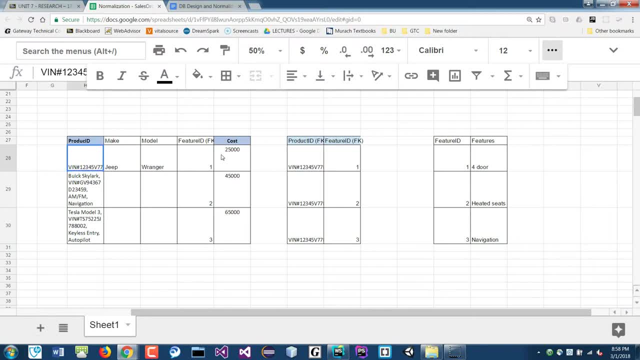 is the number of a reference, this single car, this table here. so this is a many to many relationship, but you still have to make sure that this is still, uh, normalize, Because we don't have the foreign key. What about the primary key right? 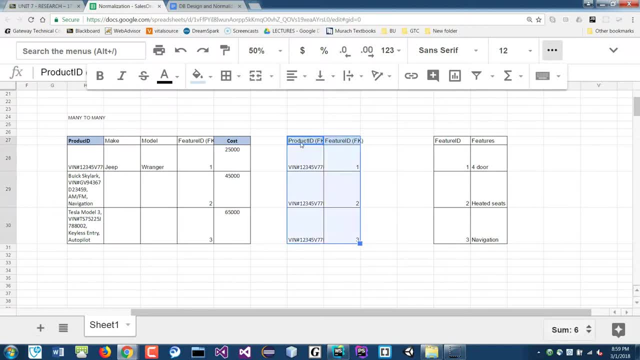 So you could have something like this. You could build something like here. I don't know car feature ID as the primary key. 1, 2, 3, just to make sure they're unique, right. So this could be the primary key. 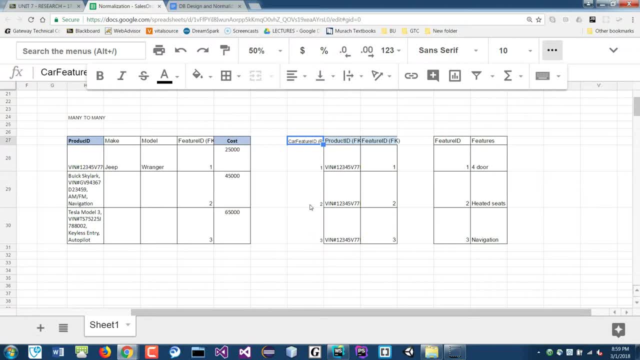 You could do that if you want. So you add a third column. If you want to do that, you can add additional information there as well. You can put the cost based on each feature, So you can have a cost column here, And then the door could be like whatever, $10,, $100, whatever. 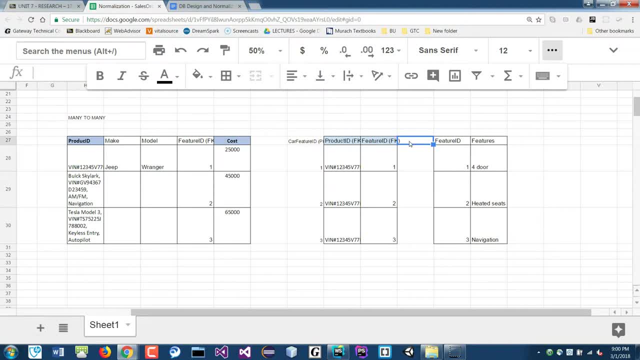 For each feature. As soon as you don't have it, then you can make this 2 as your composite key, because they are unique, right, They'll always be unique. In this case, it's the last digit makes it unique, because you're not going to have, you know. 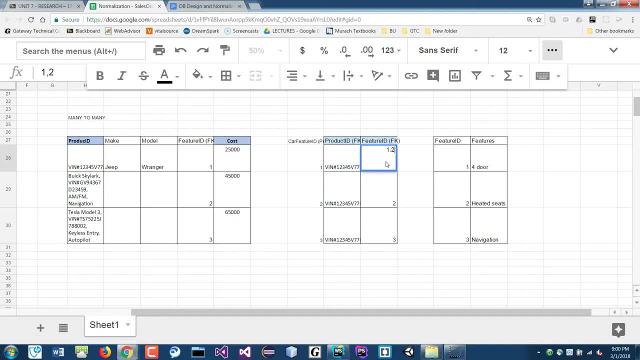 the same car has like 1 and a 2 here, right? You don't have that. It's always going to be just 1, based on the foreign key, So it's unique. So therefore, you can also make this as your PK. 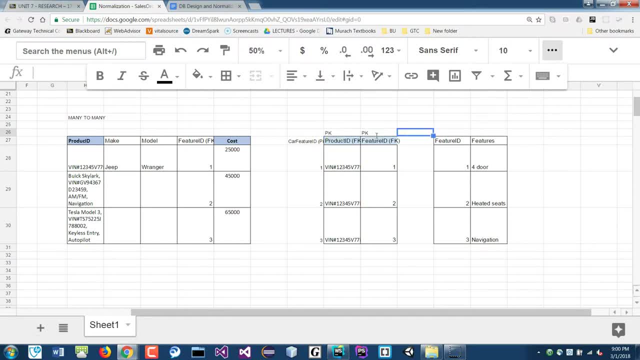 And then this is PK. So you have a compound primary key And there are also foreign keys. okay, to a different table. So for the homework, are we building these out in a spreadsheet like this or are we actually creating the tables in the spreadsheet? 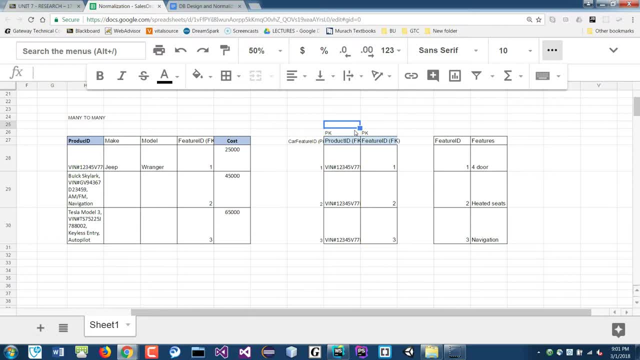 You would do both. You can draw it out by hand if you want. That's okay for the design part. But also, once you do that, then I also want you to go into the study and build a table and then the foreign keys. 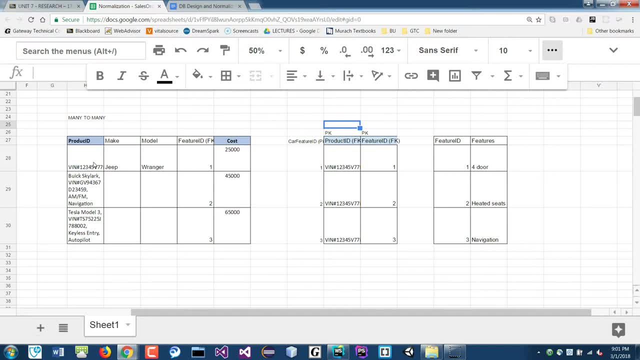 and then also generate the ERD. okay So, And in the 1,, 2,, 3 order, to show you the evolution: Yeah, The third normal form. Yes, So, the first normal form, if you want to break out into different tables, as long as they meet their first. 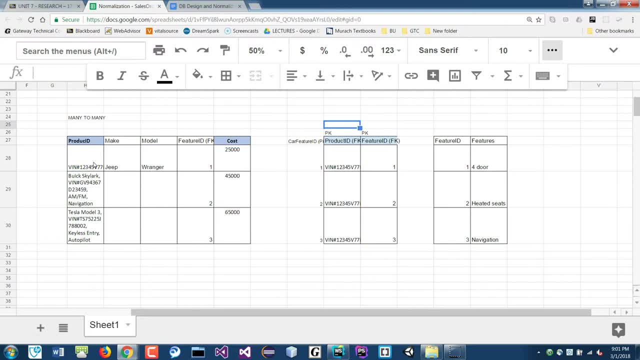 normal form. leave it at that. okay, Don't paste a third normal form in there. In this case it's okay because if you, you don't want to do that. If you take this alpha example, then that's already part. 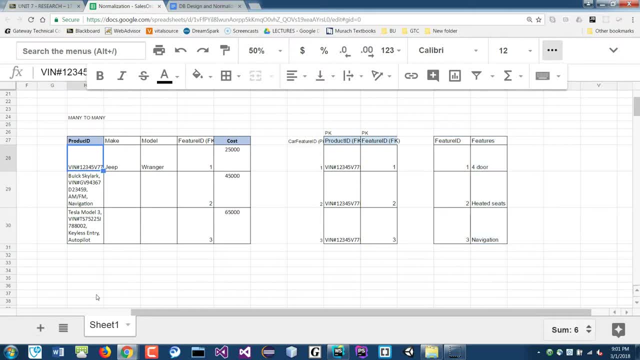 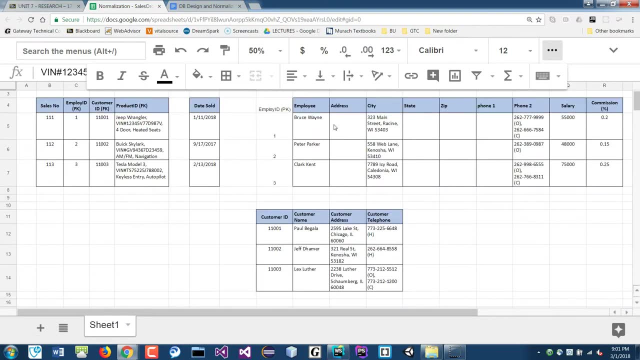 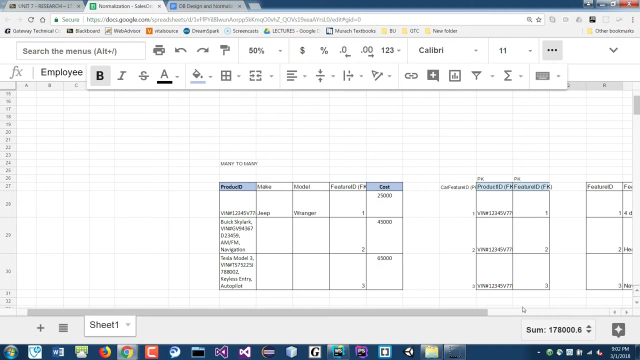 of it, then that's fine, But I should see your table in the first normal form, like we saw up here. So this is the first normal form, So this is completely fine, Okay, Okay, So I hope that I make a lot of sense here. 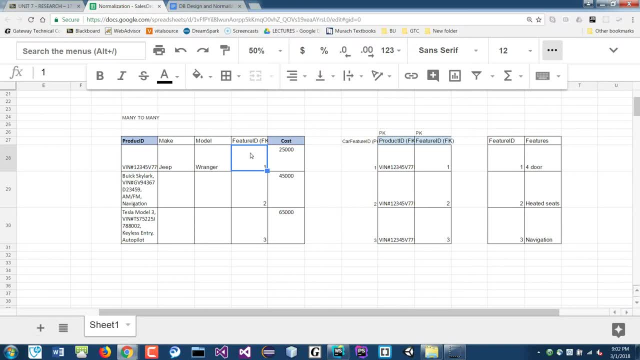 So every time we have Something like this way, you always want to think: can a car have that many features? Can one, can this feature be applied to many cars? If that's true, then you have. you need a junction table. 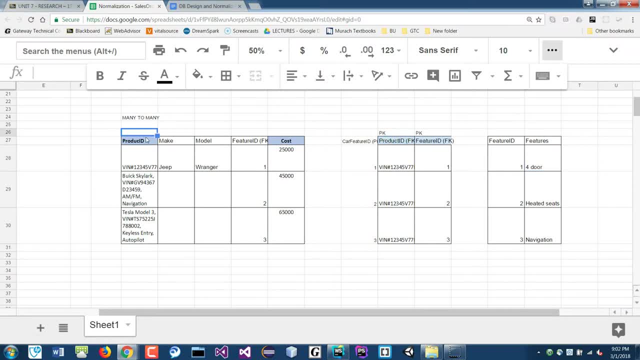 And the junction table always take the primary key from one table as a foreign key and then the other foreign key will be from the primary key of the other table. okay, And you combine those together and then you have a a many-to-many relationship table. 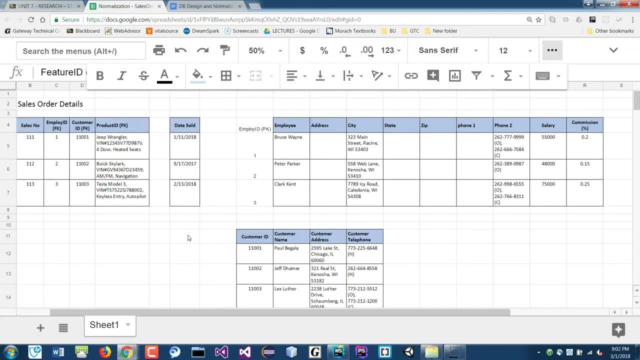 Okay, So we got that. So, and then we have the product ID. so this will be like the VIN number, right For each of these, for each of these cars, And they'll be unique because each car has a unique ID. 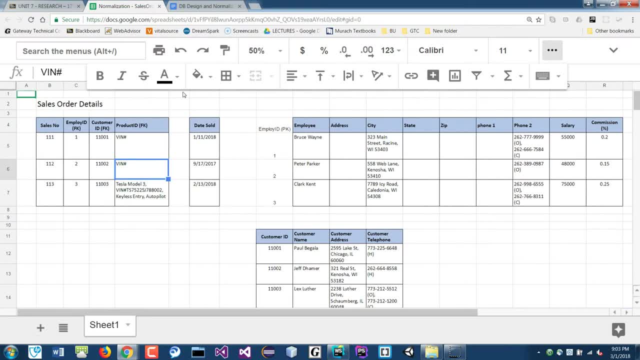 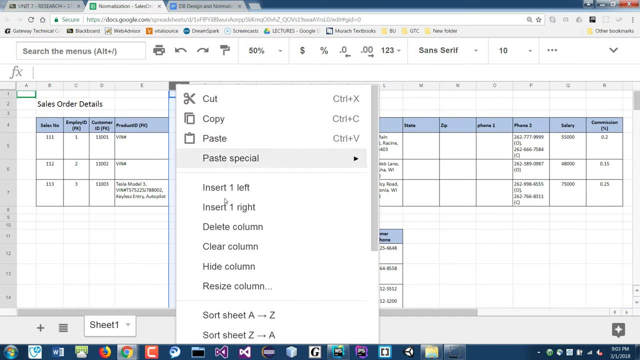 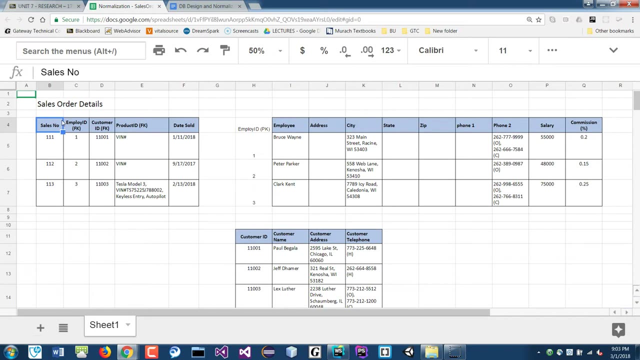 and so on, And then the date sold will be will be fine part of that, And we can combine this together. And so now this table is in it's good Qualify, it meets the first normal form, And so I'll do this and all of these are, so we are good. 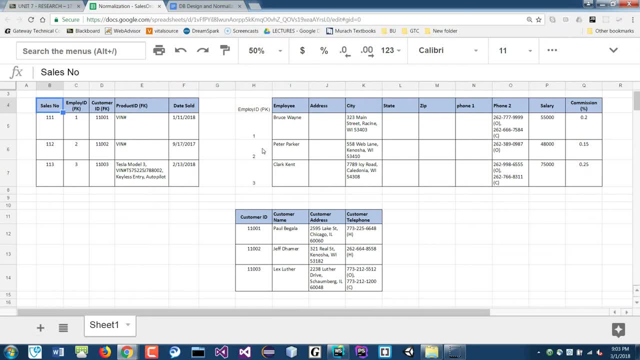 We're just kind of doing this and the reason I ask is because I'm trying to make sense of this. A VIN number actually has most of that information in it. This information, Yes, Right, So a lot of the VIN number. there's a lot of that information. 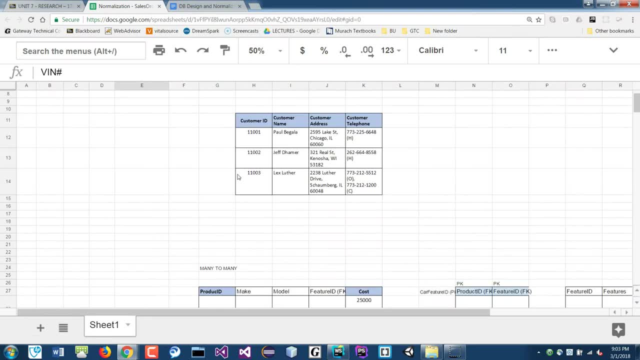 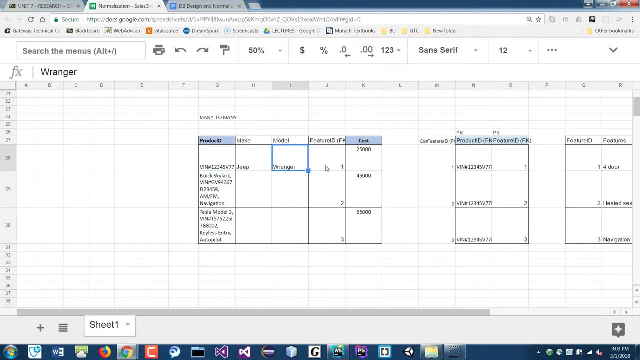 Mm-hmm. So the VIN number? right. so that's where you put in the product's information. here The VIN number tells you that it's a Jeep, it's a Wrangler, has these features for this car. Well, what I mean is the number itself. 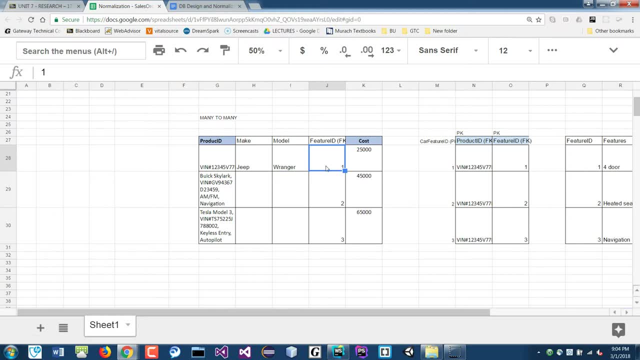 Mm-hmm, The VIN number on your car. if you go out there and take it down and you look it up, Yeah, It will give you a list of quite a bit of information in there: Features, the color, what it was made, the engine size. 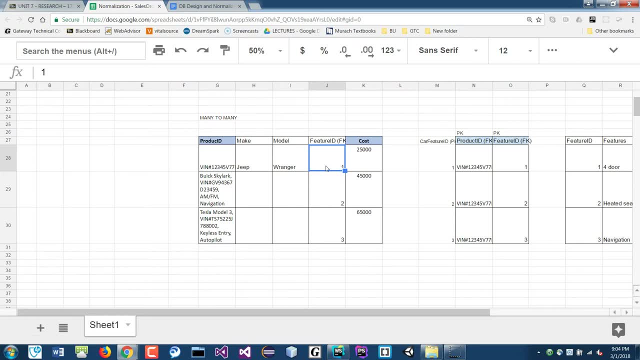 Right, Encoded in that number, Right. That's what we're showing here. How do you see that information? Mm-hmm, How do you see that information? It's a Jeep, it's red, it's built in 1945, for example. 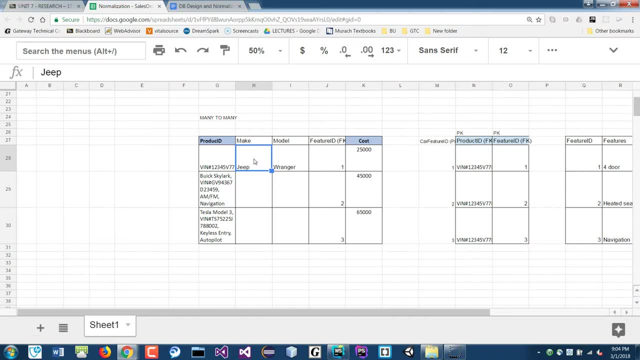 How do you know that In the VIN number? So if I just give you this VIN number, can you tell me it's a Jeep Mm-hmm. I don't know if I can fit it in the model, but I can. 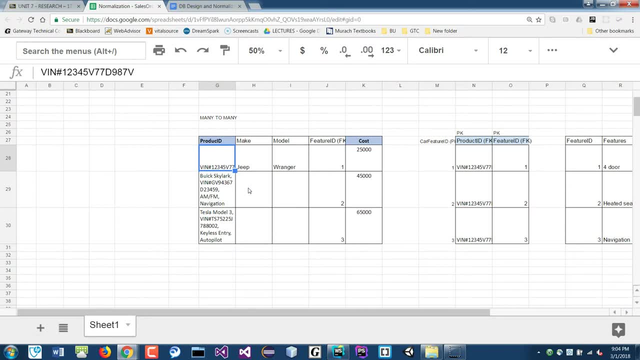 No, you can take that VIN number and look it up in the table. Mm-hmm, Right, So you need it. It's down in all the pieces of water where it's falling Right, So somewhere you need. 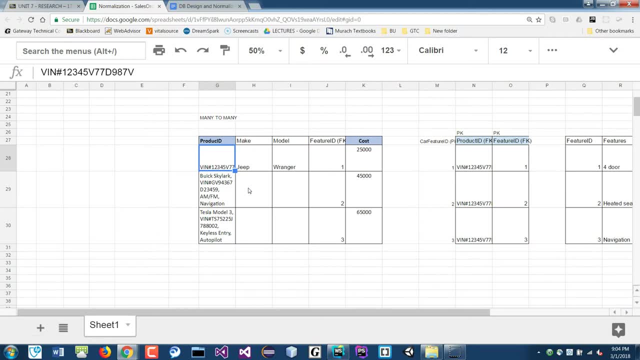 It's still in that table, Mm-hmm, In the great scheme of things. Exactly That's why you say all these are dependent on the VIN number, right? Every column must depend on the primary key. That's exactly what you just said, right? 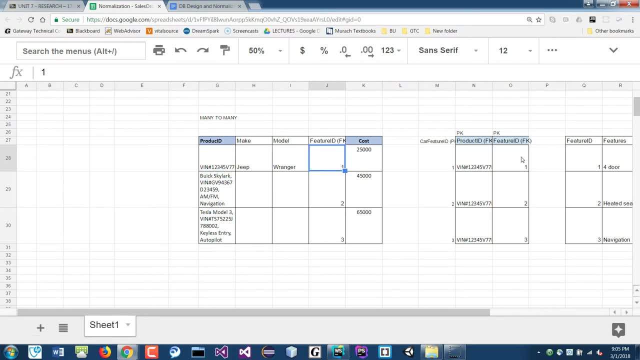 Mm-hmm. So the Jeep- it's a Wrangler, it's a- has this feature, has this year, has this engine size, For example. all those are dependent on this Jeep VIN number here. But if you just give this VIN number, like you said, if we give this VIN number you can look it up. 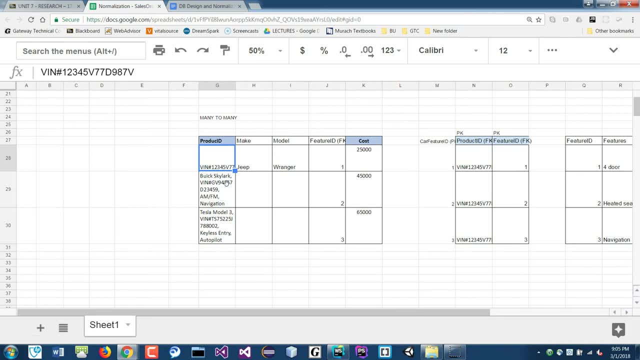 and you can tell exactly what that car is. That's exactly why you built this table right: to make it very unique. But how do you see those is the actual data. We don't see that, So you have to put in the data here so we can get those data out. 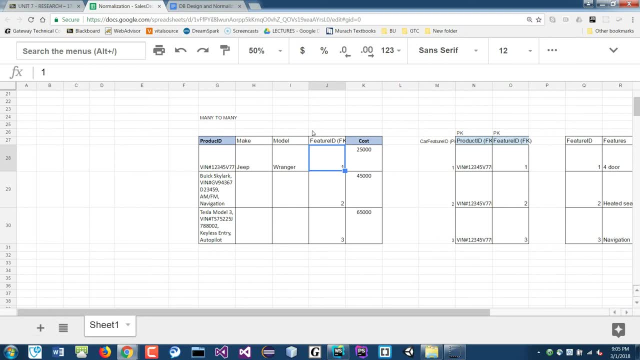 But your point is- it's made a pretty good point And it's exactly why you have the entity that is unique about only one object. Okay, So, for example, I wouldn't put like, I wouldn't put something like a driver, for example, right. 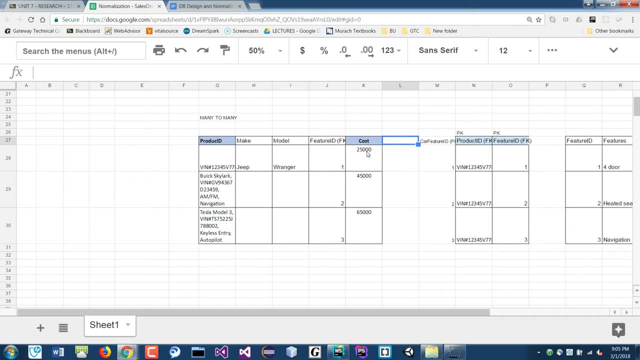 A driver wouldn't fit in this category, Because this Jeep can be driven by anybody. Okay So, And the DMV would have that related in another table. as a registered driver? Yes, So, if you have a driver, then I mean the driver's license number would be your unique ID. 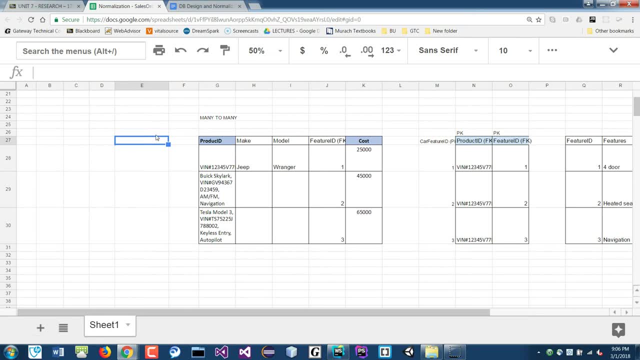 And on the table it's the driver. Yeah, So if you have a owner, that's different than a driver table, right? Yeah, So one car can be owned by one owner, but it can be driven by many drivers, So you have that relationship too. 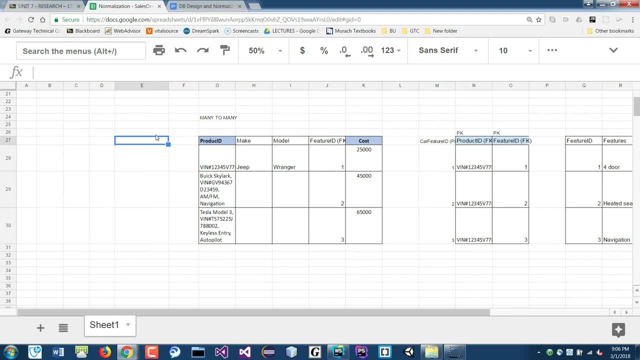 So, when you build this table, expand it. you see, oh, I have an ownership table, I also have a driver's table. if you were to, let's say, work for a taxi company, right? So yeah, so you can see how you can break this out. 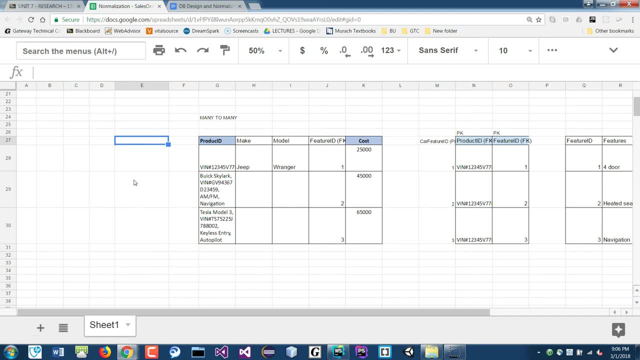 You can break it out into a lot of tables and they're related in those situations. And then the- I mean above all. this is just basically, you are trying to solve some business problems. That's all about building databases. Really, you build database based on business problems. 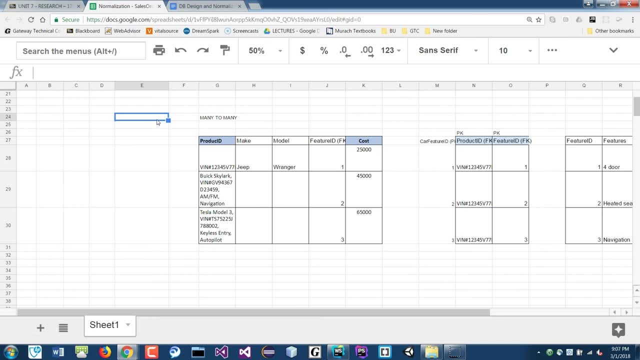 And you'll see that if you go into becoming DBA, for example, you go into deeper in database design. that's exactly what you do. You have to come up with a list of business issues and how do you solve it, And then, from there on, build your database based on those to meet those business needs.